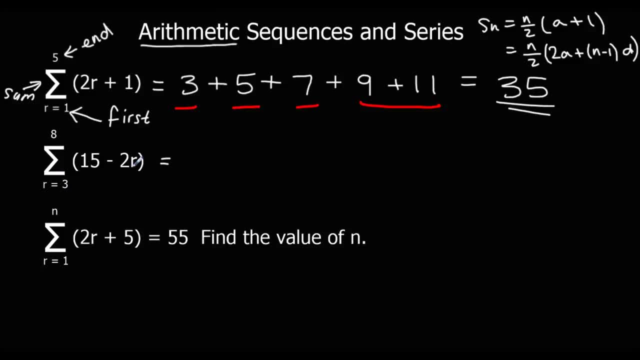 So if we write them out, starting with r is 3, so substituting it in 15, take away 2, 3s, 15, take away 6s, 9, and then 15 take away 2, 4s. 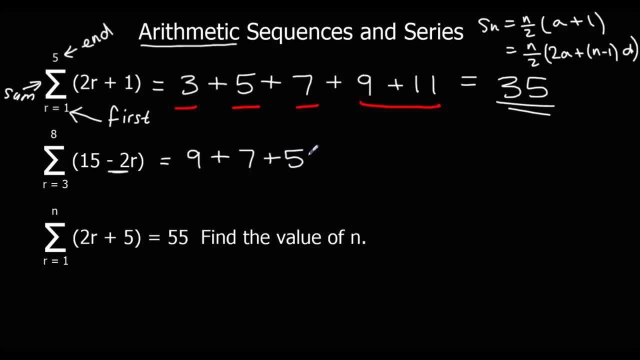 This one's going to go down in 2s, So 15 take away 2, 5s. 15 take away 2, 6s. 15 take away 2, 6s. 15 take away 2- 7s. 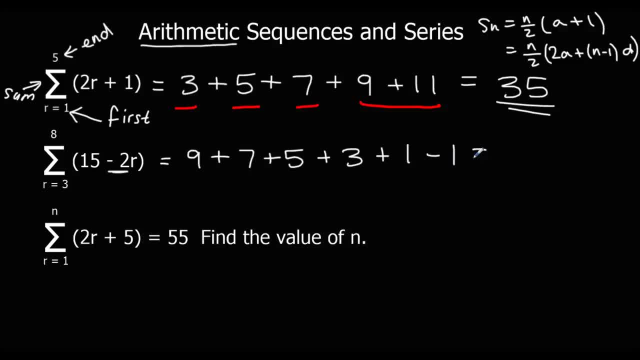 and 15, take away 2, 8s be minus 1.. Then we add them up, so that's 0,, 10,, 19,, 24.. Okay, the third question is different because they've told us what it adds up to. 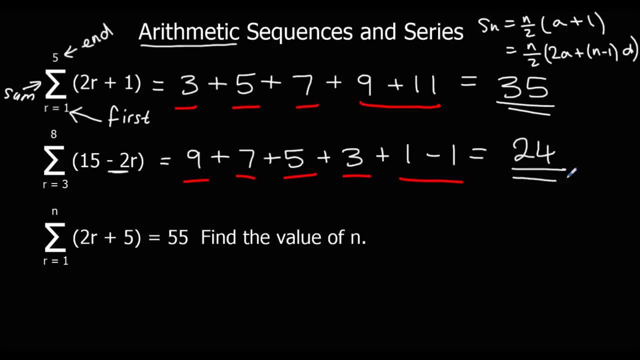 and we've got to work out n. So we've got to work out what the end number was. Again, two ways of doing it. We could substitute into this the formula. we'd have to work out a and d first, And to do that we'll just have to work out the first two terms. 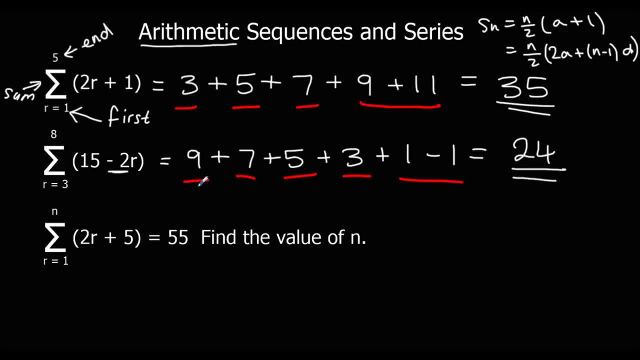 But yeah again, probably just as easy to write them out and find out how many numbers it takes to get 55, because there's not going to be that many numbers until we get to 55.. So the first term, 2- 1s, starting with 1,. 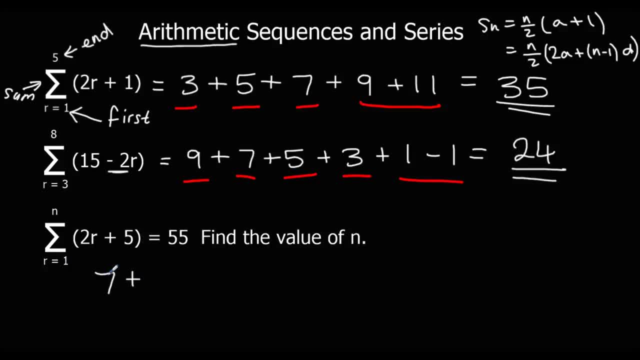 2 1s plus 5 is 7,, and then 2 2s plus 5,, 9,, and so on: 2 3s plus 5,, 2 4s plus 5,, 2 5s plus 5,. 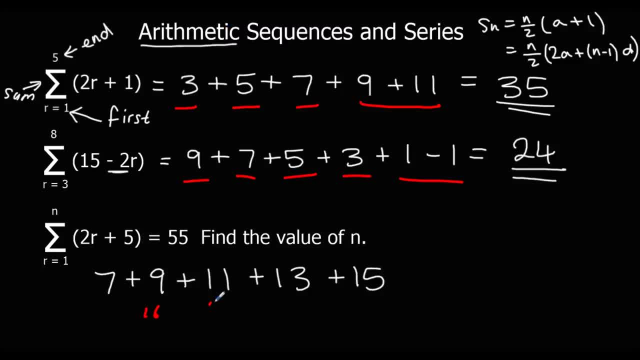 and I think that's 16,, 27,, 40,, 45. So n is 1,, 2,, 3,, 4, 5.. n equals 5.. We could have used the sum formula. It would give us. 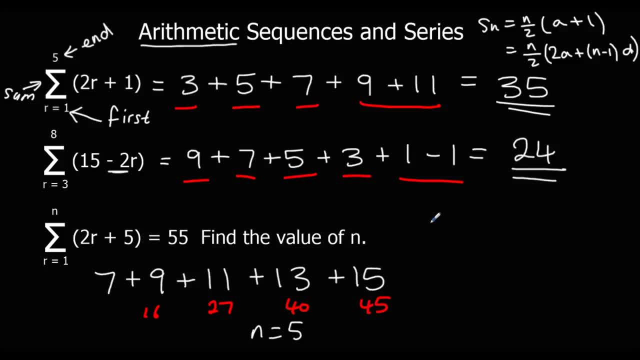 it's a quadratic to solve, So let's have a look at doing that. So sn equals n over 2, 2a plus n minus 1d, And we know a is 7, and the difference is 2.. You may have to work out the first few terms to figure that out. 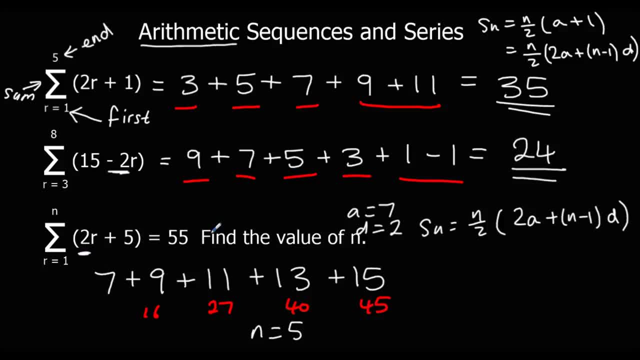 That's going to be the difference, Like the nth term, the thing with the n, the thing with the r is the difference, Or you can just write out the terms. But yeah, you might have to write a few out to find out. 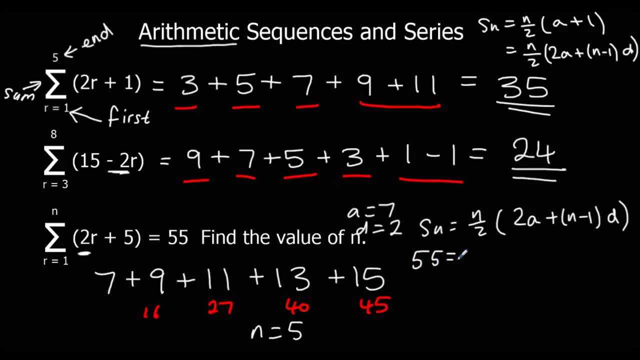 So the sum is 55, and that equals n over 2 times 2, 7s plus n minus 1 times 2.. So if I get rid of divide by 2 by times in both sides, by 2, first, 110 is 2,. 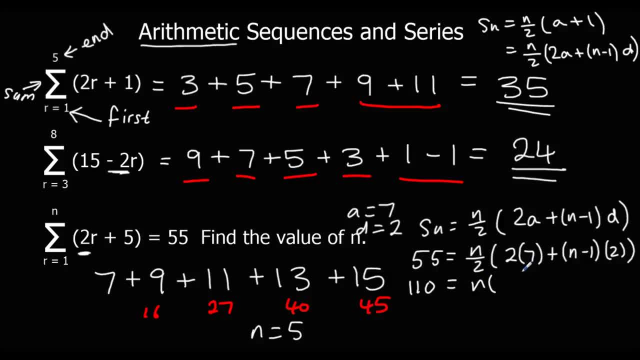 and then I've just got n here, now 14, and expand the bracket at the same time to n minus 2.. So 110 is n times 14. take away, 2 is 12 plus 2n, And then 110 equals 12n plus 2n squared. 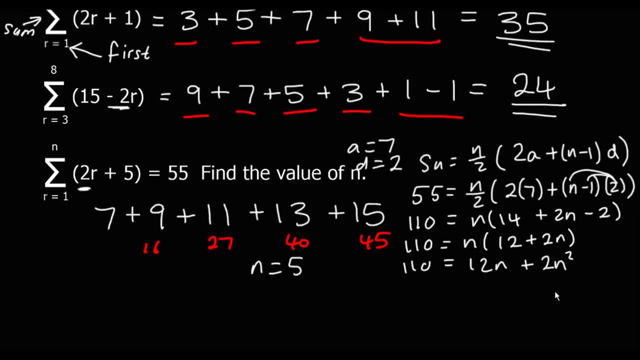 We've got a quadratic. So to solve a quadratic we need to make it equal to zero, And I'm going to write the n squared term first, then the n term minus 110.. So I want to factorize it First thing I'm going to do. 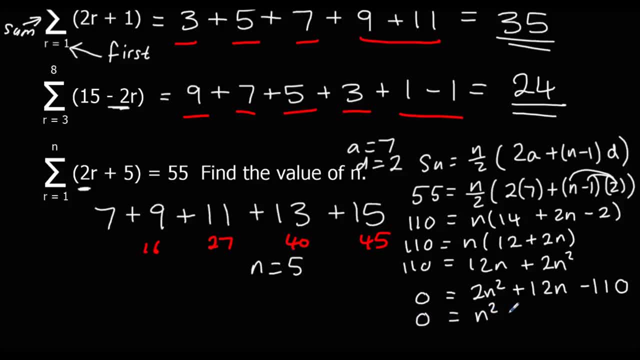 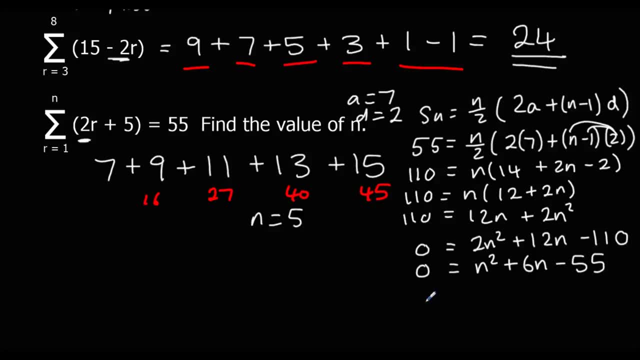 I'm going to half it. They're all even numbers: n squared plus 6n minus 55.. And then I'm going to factorize it. So we're looking for what multiplies to make 55, adds to make a 6.. 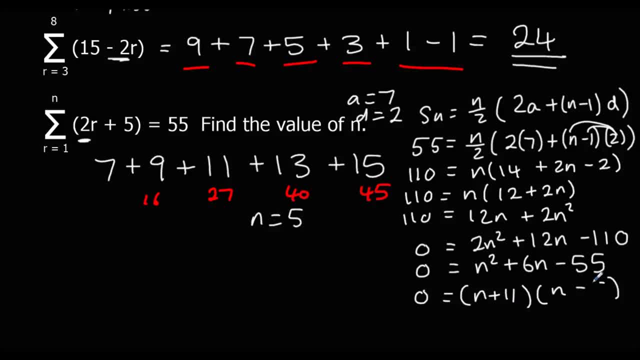 It's going to be 11 and 5 plus 11 minus 5.. So that give me n is minus 11 or n is 5 and can't be a negative, So it has to be 5.. So I think it was probably easier to write out the numbers there rather than solving the quadratic. 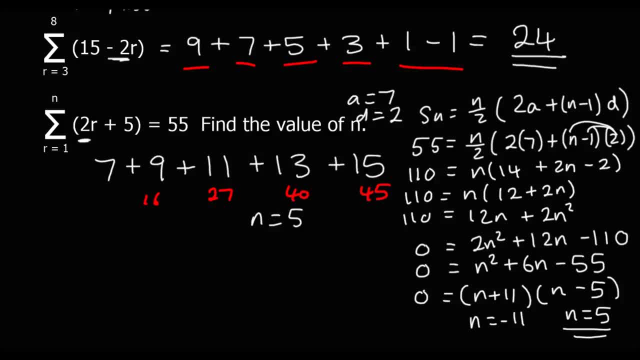 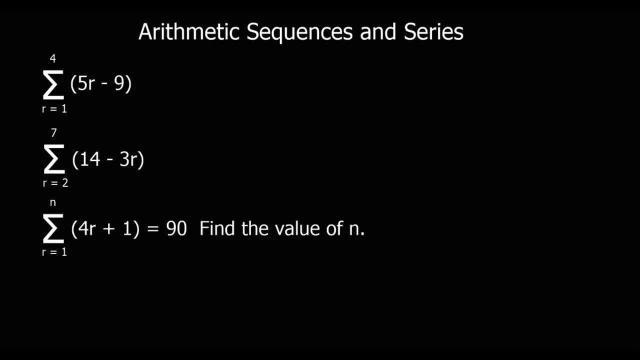 But both methods work. Both methods work. So here's a few more questions. See if you can give these ones a go. So see if you can figure out the sum for the first two and then n for the last one. OK, so we've got. starting with r is 1, going up to 4..